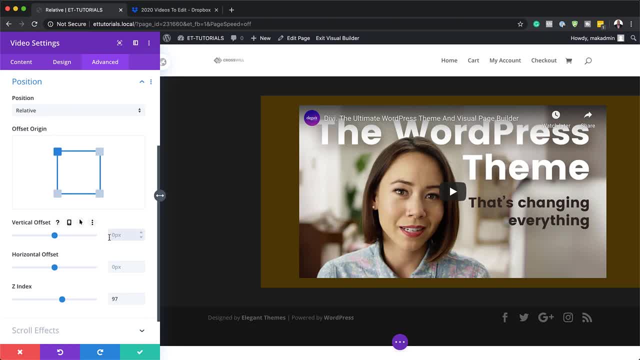 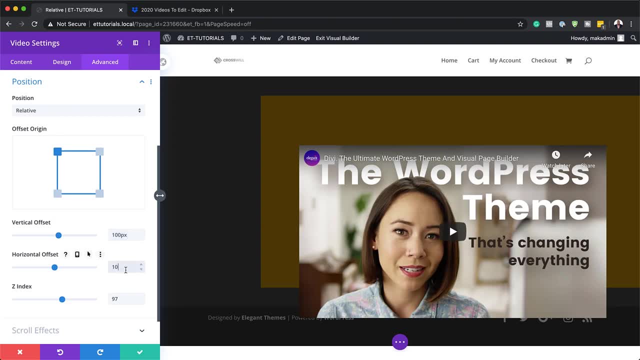 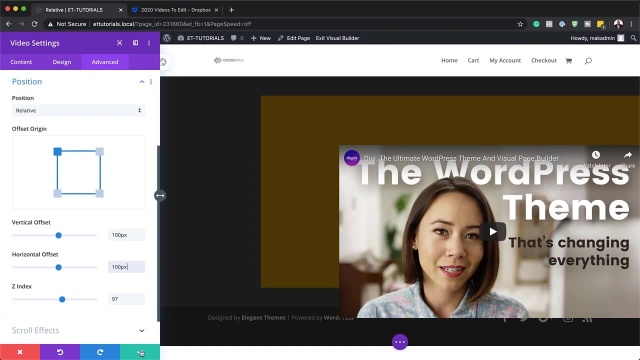 which is top left In this example, you can add a specific value, So let's say a hundred. So you can see, there, I've just moved my video and I can offset it to the right as well. So there we go, A hundred as well. So this allows us to pretty much have this at the right position that you want. 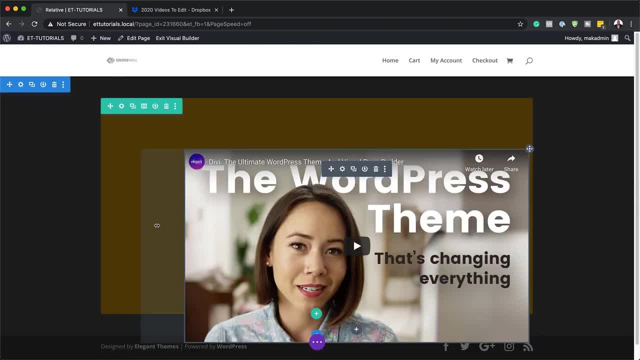 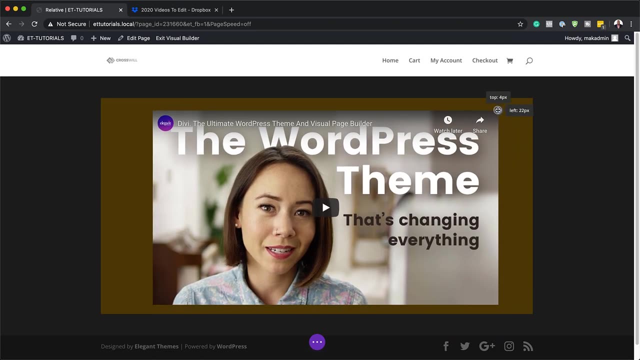 Now another quick thing I also want to show you is, once you've added your relative positioning, if you close that settings panel, you can come over here and hover over and see that you now have this little icon which allows us to specifically position this wherever we want. 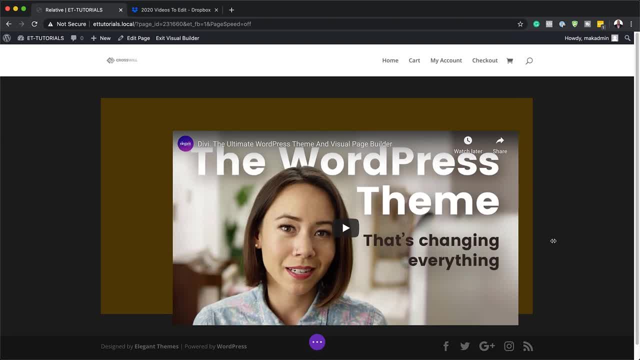 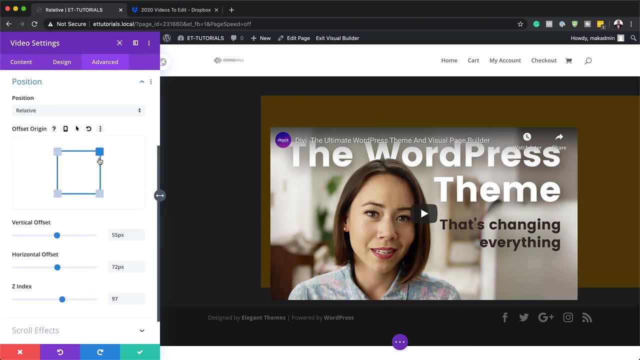 So that's the advantage of this: You can do this visually. Okay, Now let's say you want to use the top right offset. So what you could do is, again, you can come back over here, click on position, and then you go over here to the top right And then you 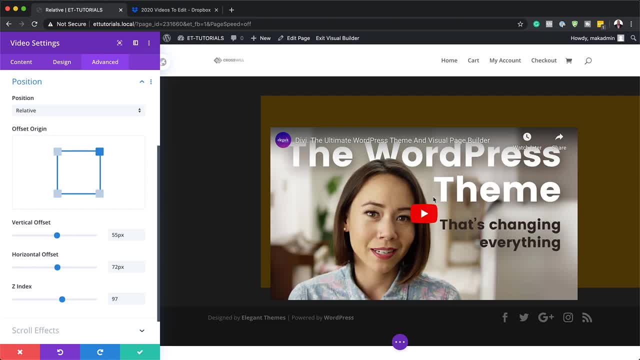 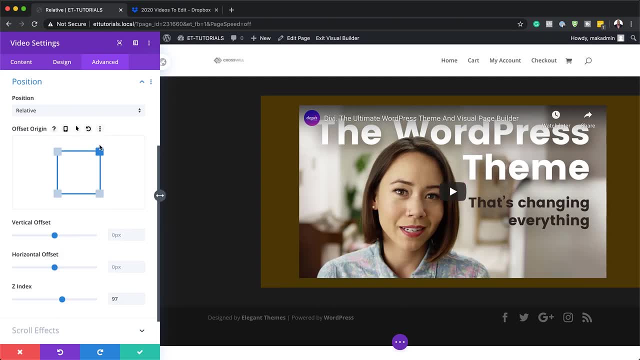 can use this as your offset origin. So this will be your offset origin and you can also play around with this if you need to as well. So pretty much you can choose any origin and then apply your offset values. So again, let's say I want to use the bottom here. I can choose bottom and then 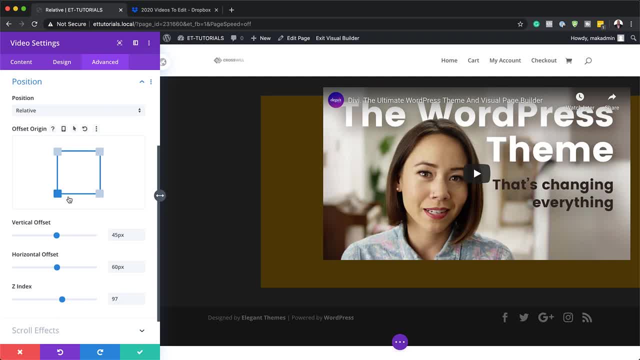 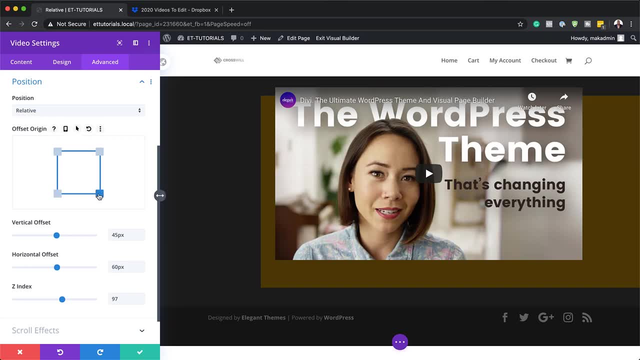 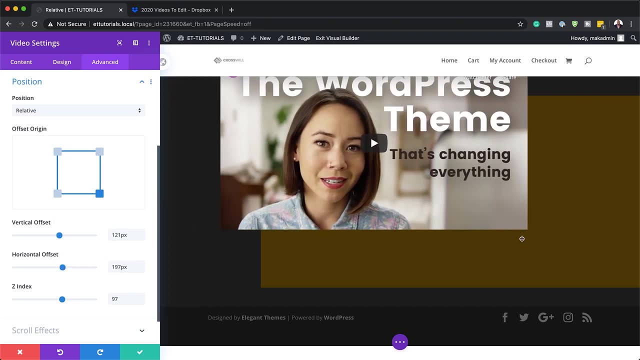 I can move this wherever I want. So, as you can see, this is the origin. So pretty much this bottom left here is the origin that I need to offset with. If I come over here, it changes the origin as well. Look at that Now. it can go up and down, but using that position there as the 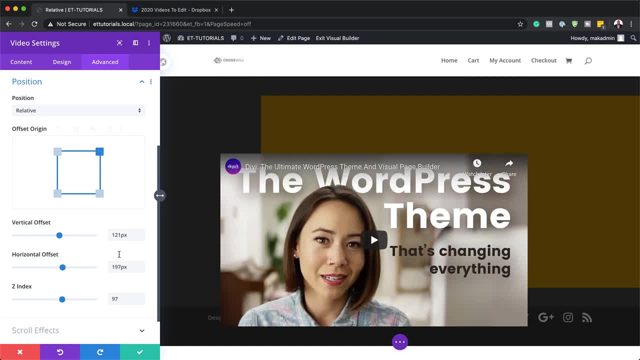 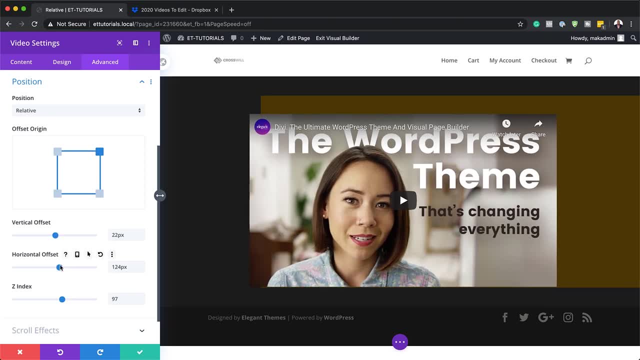 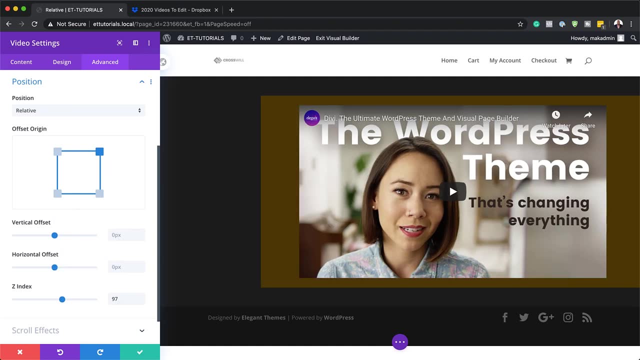 origin, which is the bottom right, And then, of course- I've done this already- This is the top left. I mean top right. sorry, Sometimes I get this top right, top left, uh, confused. All right, So I'm just going to reset this, now that we know how to use this Now with relative. 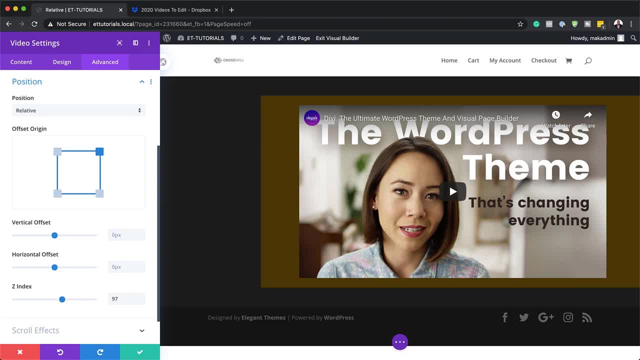 positioning. the actual space of the element remains in its original place after the element is moved using the offset. bottom left, top right. The elements new position doesn't move or affect any of the spacing of the rest of the elements on the page. This basically hovers over the other.